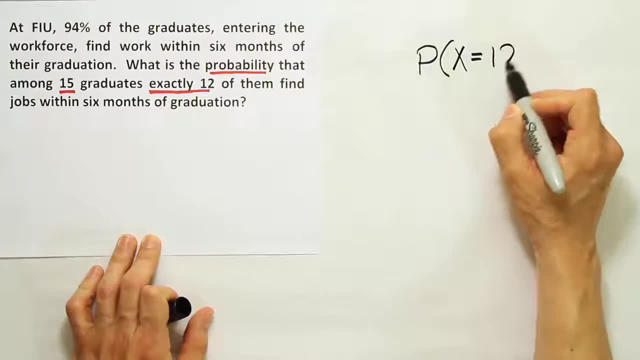 that the number of people who find jobs x is equal to 12.. So we're going to let x be the number of students who find jobs. All right, Then, from there, what we want to do is to fill out the binomial formula. if that's what, 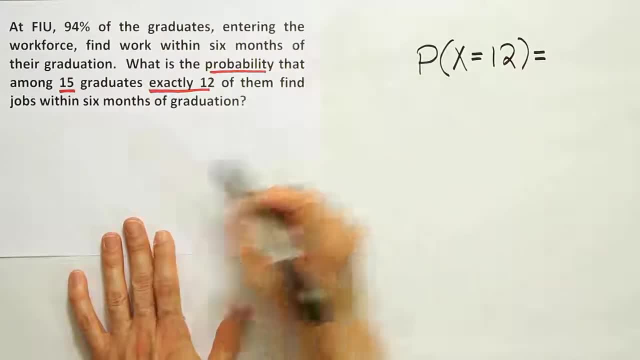 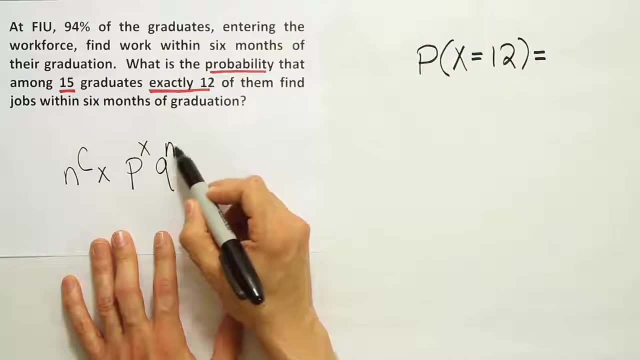 we think it is. So. the way the binomial formula works is: we want to fill out this formula right. We want to have n choose x, p to the x power, q to the n minus x. Okay, So our n here is 15.. 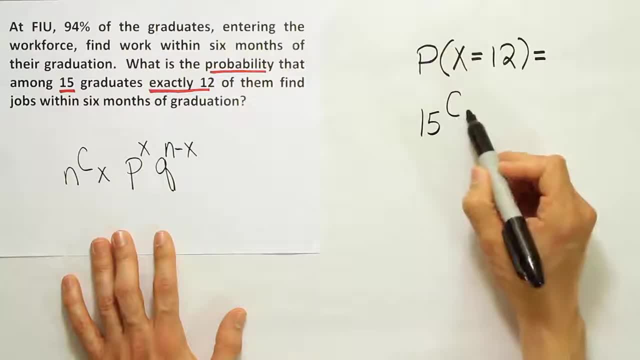 There are 15 graduates being looked at. We want to choose 12 of them to be the ones who find jobs. Then we're going to have the probability someone finds a job. That'll be 94.5.. So we're going to. 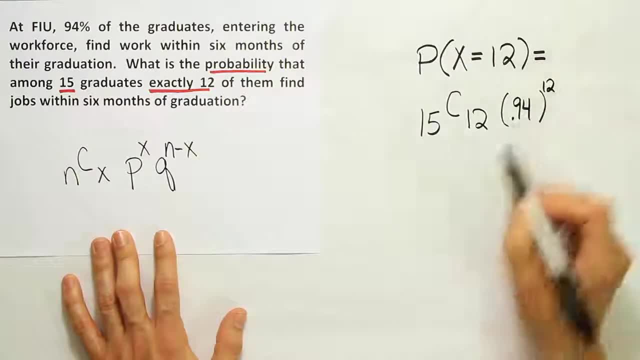 put the 12 on the 94%, There'll be 12 of those people, So we'll put the 12 on the 94%. If 94% find jobs, we need the complement of that, or in other words 0.06.. In other words, 6% that do not find. 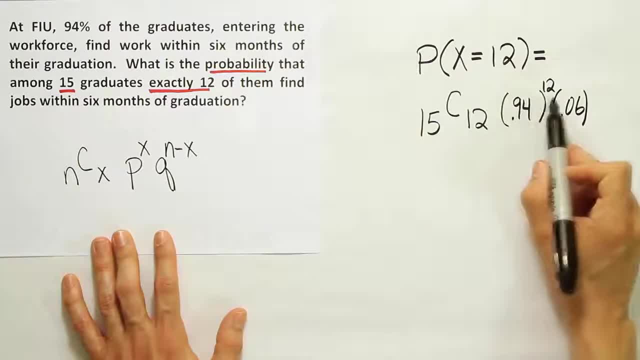 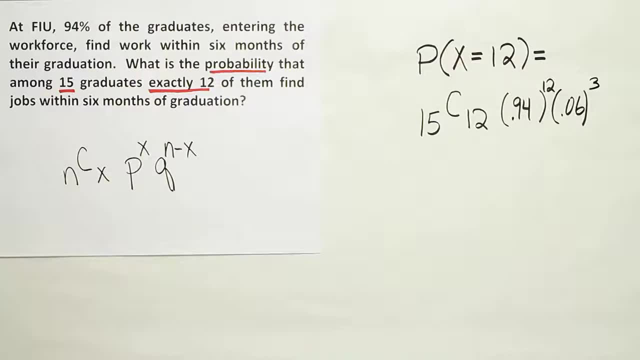 jobs, Then we need the complement or the leftover amount from 15 that won't find jobs. If 12 get jobs, the remaining three do not, And that should be our solution for the problem. The rest of it is just calculator work, So let's go ahead and do that. 15 choose 12 can be worked out pretty. 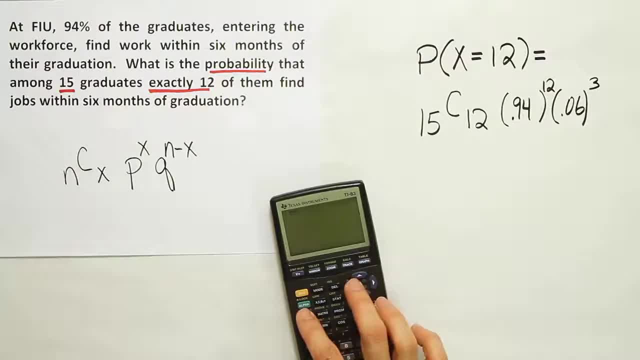 easily by hand, But we're going to just go ahead and do that in our calculator, So we're going to use our calculator to speed it up. That ends up being 455.. And then we multiply by the remaining two quantities, And so that would be times 0.94 to the 12th power, times 0.06 to the third. 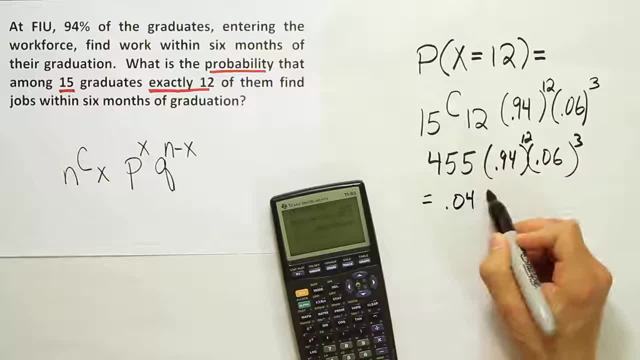 And when we're all said and done, we end up with 0.0466.. So as a percent, that's 4.68%. Okay, so about a 5% or 4.5% chance that exactly 12 of the graduates will find jobs within six months of graduation?